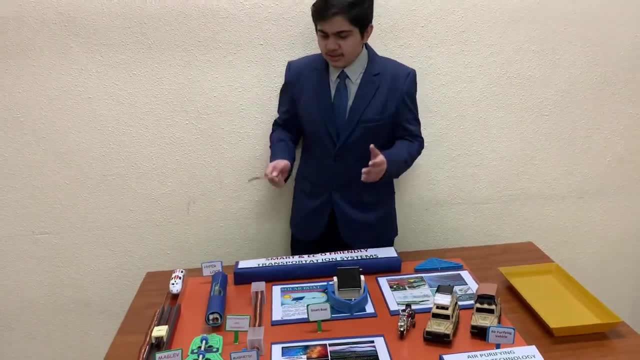 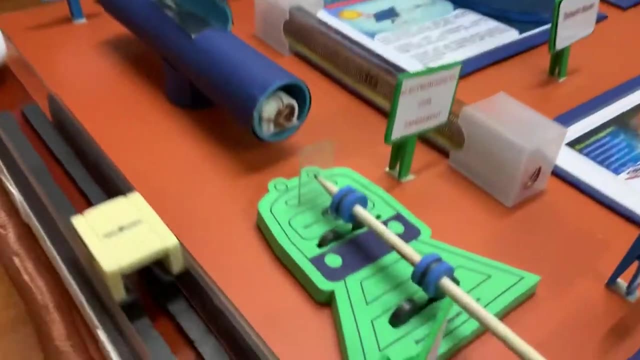 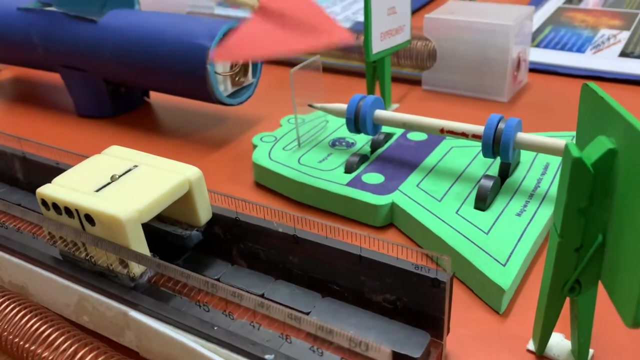 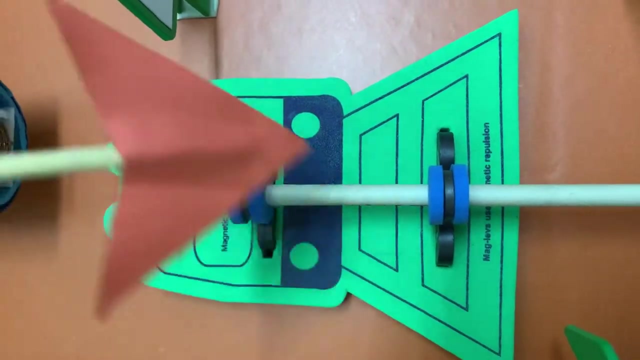 Now let's see the floating pencil. You must be wondering how this pencil is floating. This pencil is floating because there are magnets in the base And there are round magnets in the pencil as well, So the repulsive force between these magnets makes the pencil float. 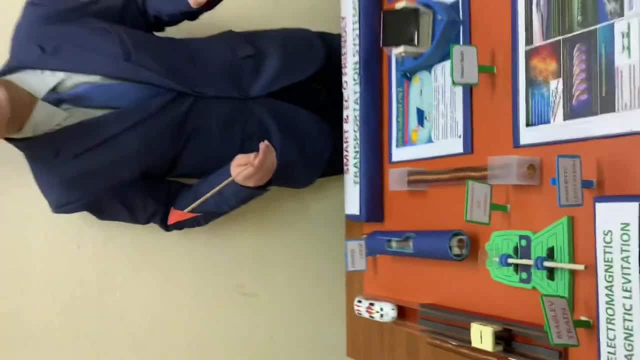 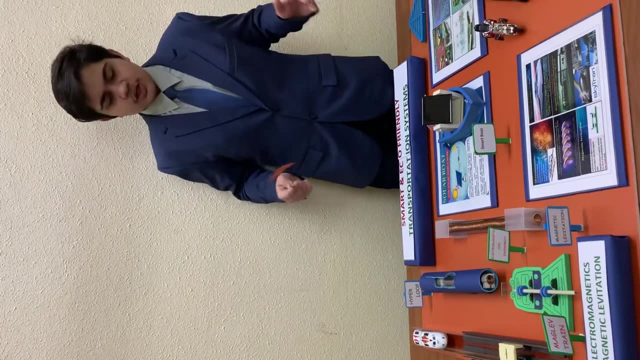 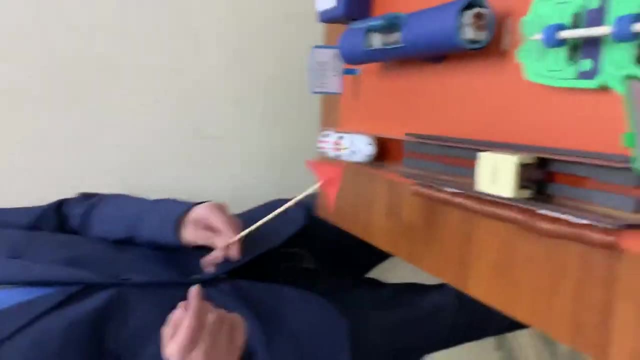 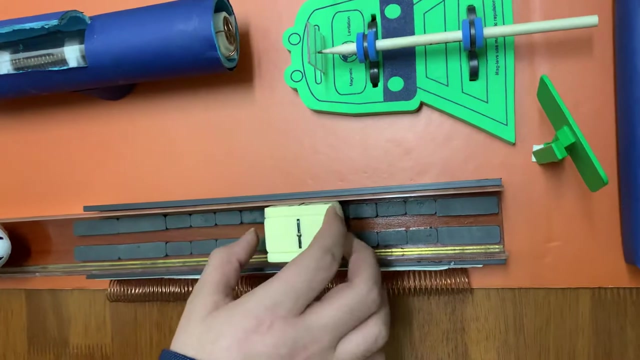 So you all must have heard about high speed trains, called magnetic trains. in countries like Japan. These trains also work on the principle of electromagnetic and magnetic levitation. I have created a prototype of the magnetic train. You can appreciate the way the train floats on the track and moves smoothly. 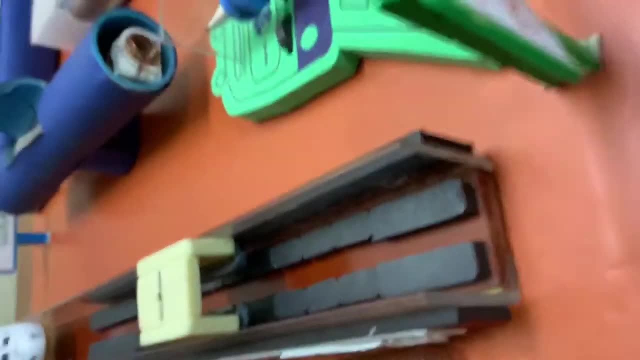 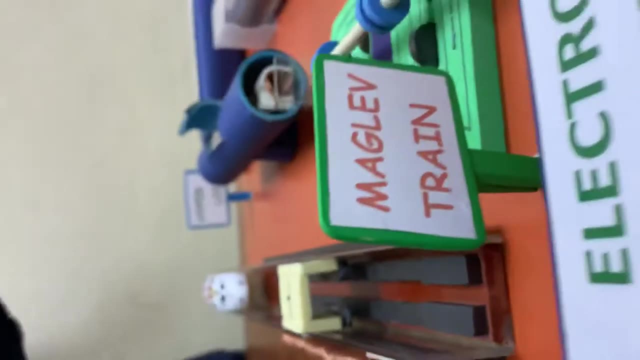 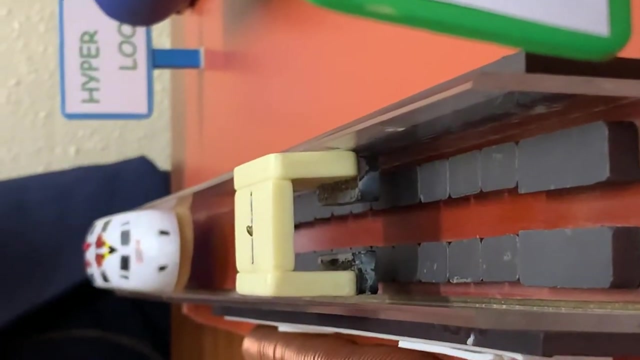 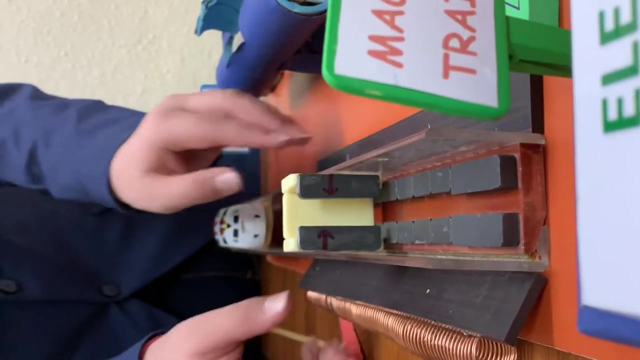 As there is no friction between the track and the train as the train is floating, So the trains are able to achieve very high speeds, About 650 km per hour. Now let me show you the importance of these magnets at the side. So as I remove these magnets, the train topples. 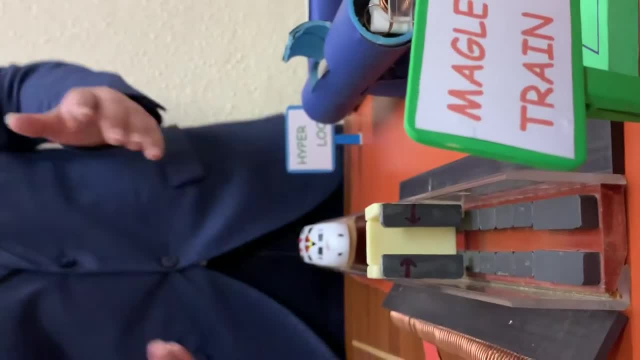 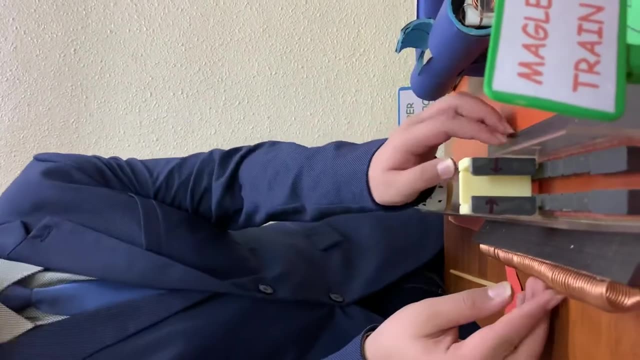 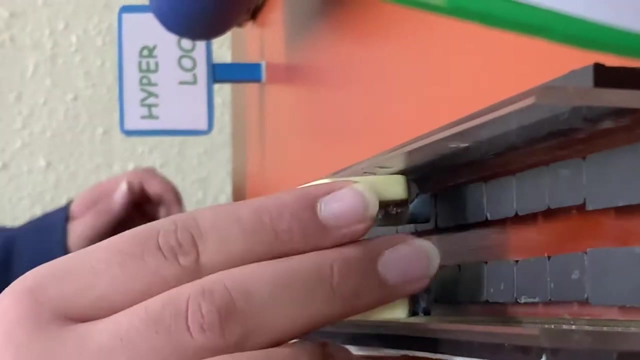 Why? Because these magnets at the side are called the lateral guidance magnets. They provide support and balance to the train on the track. Now, as I put these magnets back and place the train on the track, The train starts floating again and moves smoothly. 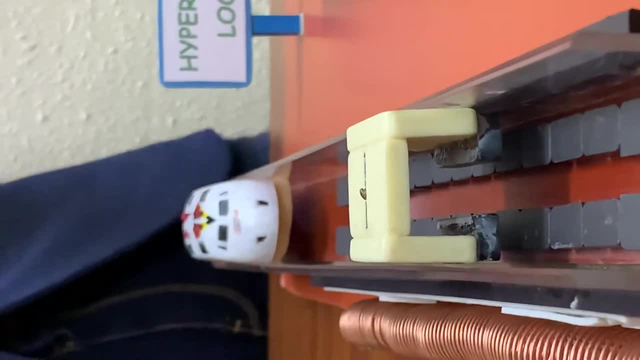 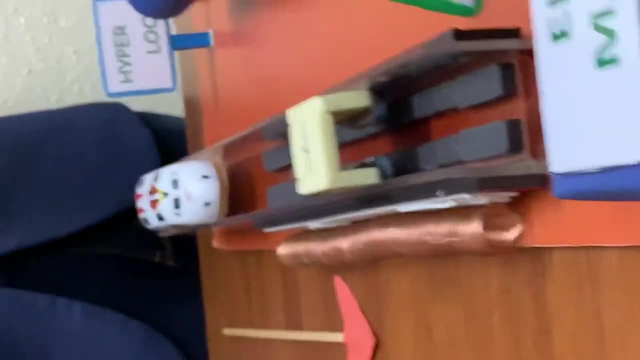 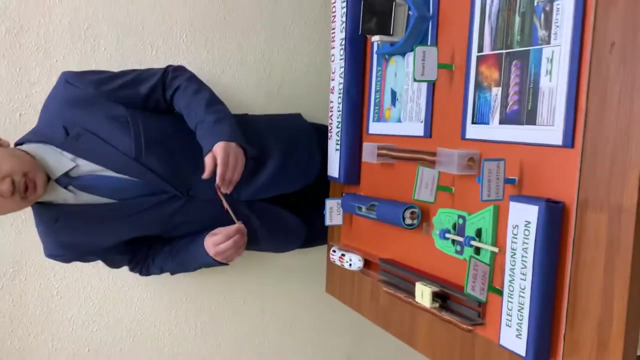 So this is the magic of magnetic levitation, And this coil can also be made into an electromagnet If the same cell with the neodymium magnets is fast through it. This is also a propulsion coil, Now moving a step ahead, Coming on to the hyperloops. 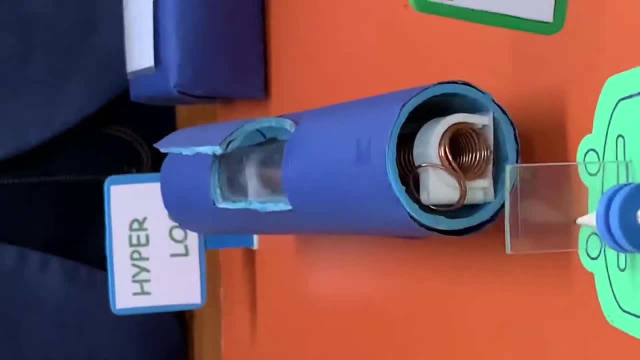 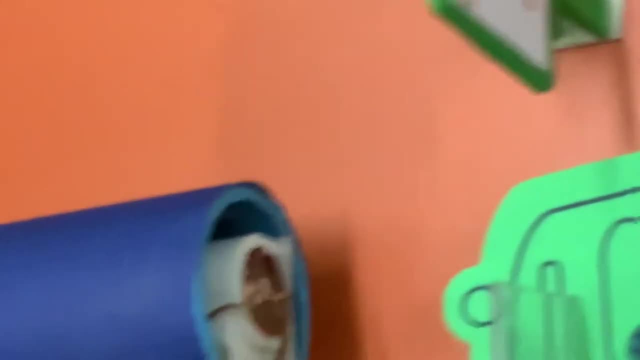 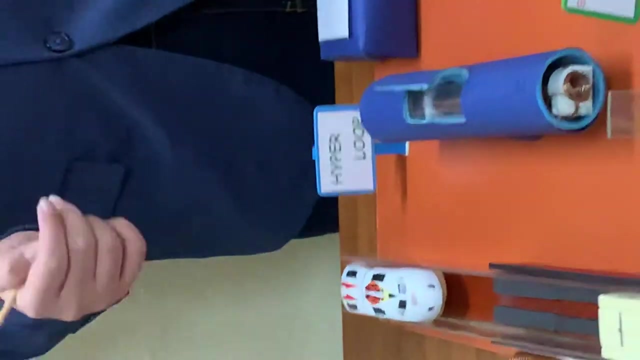 Hyperloops are also a type of magnetic train Which works in a low pressure environment to reduce the air drag. Now, as the air drag and friction works, Both are reduced. These hyperloops are able to achieve very high speeds, Even faster than most of the jet planes. 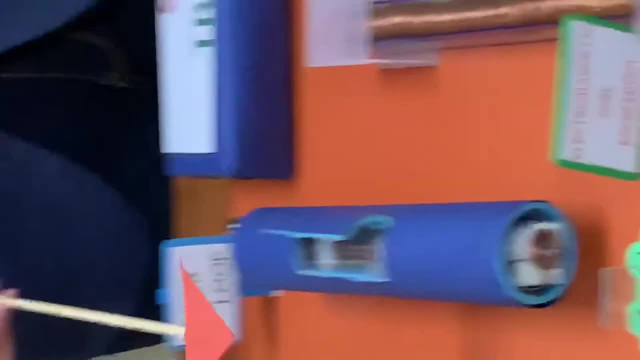 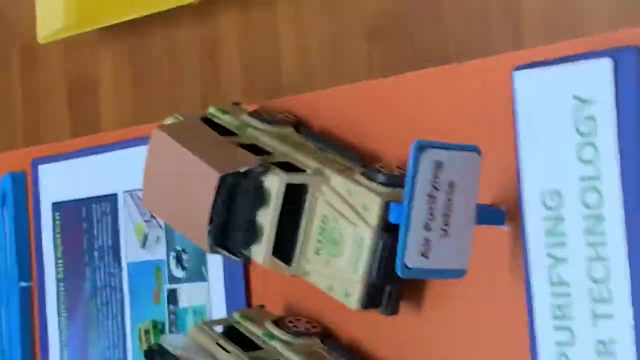 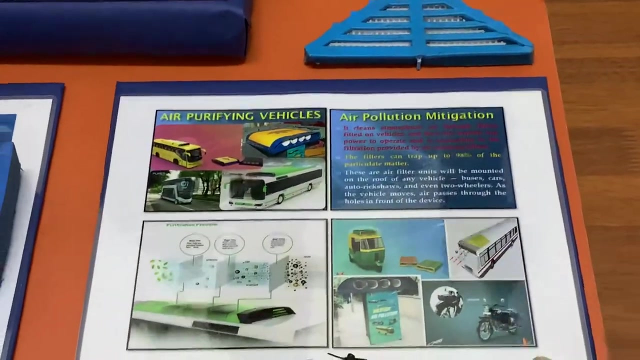 And some of them are being created in Dubai presently. Now, coming on to the air purifying vehicle technology. How can these vehicles purify air? So, with these latest technologies, Vehicles themselves can purify the air. As you can see, I have a vehicle. 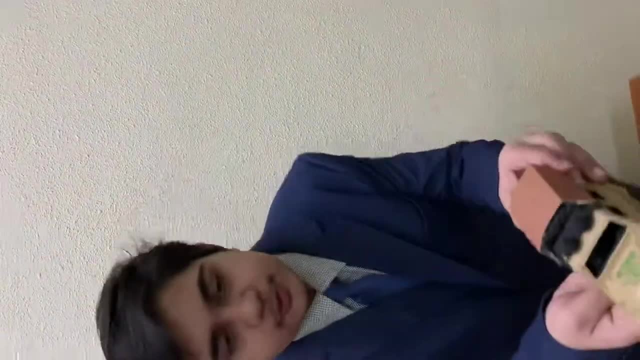 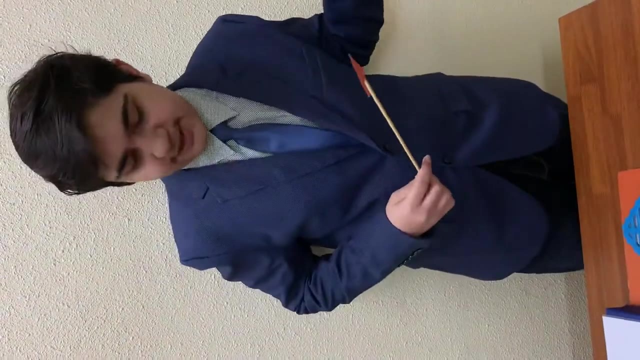 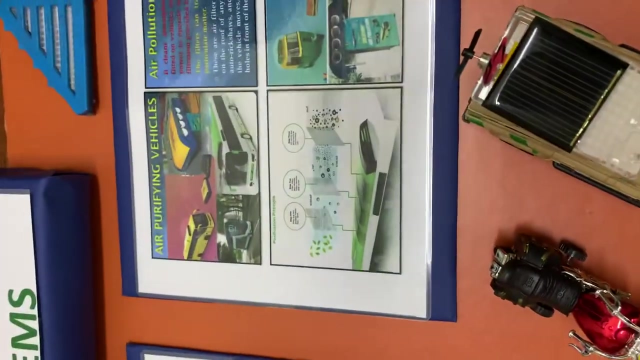 It has filters attached on the top So as the vehicle moves forward, Air passes through these filters. So when the air passes through these filters, It gets purified. This filtration takes place in three steps, Based on the materials to be purified. This is how the filter looks like. 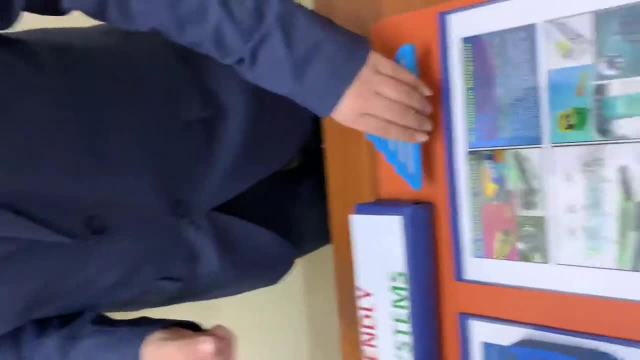 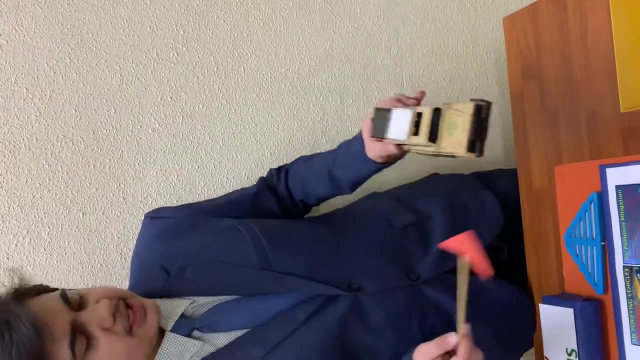 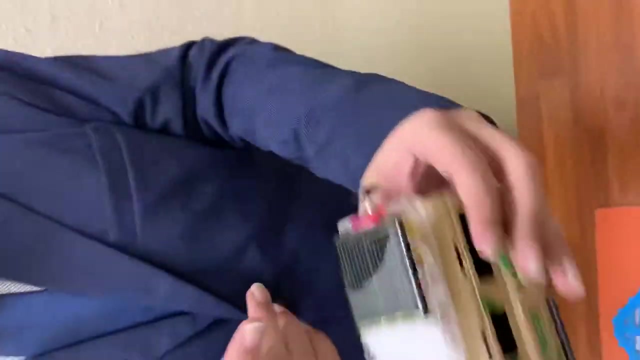 In three of its steps. Now I have created something interesting. I have modified this And created my own invention. I have attached a solar panel in this filter And an exhaust fan which can suck in the air, So even when the train 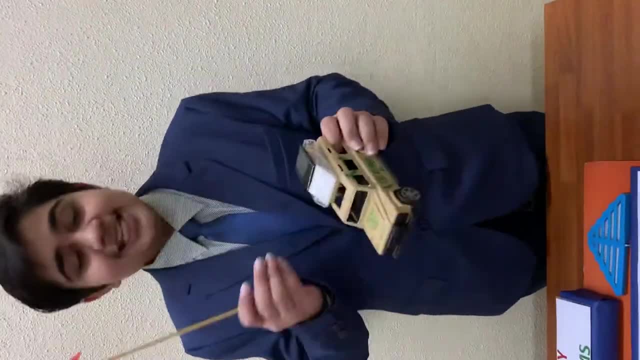 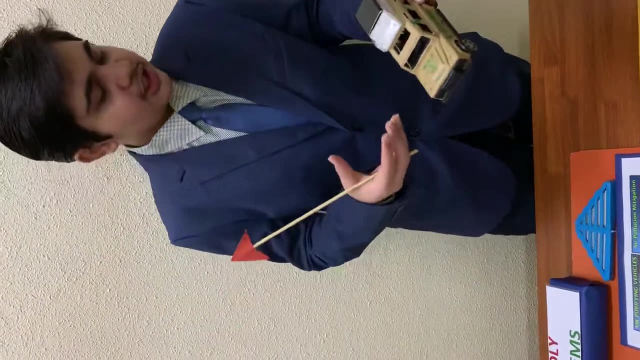 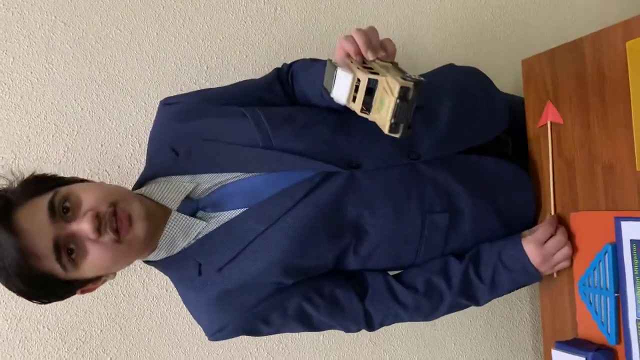 Even when the vehicle is not moving, It can purify the air, And these solar panels can even store energy in the batteries, So that it can even be operational at night. Isn't it amazing? Now let me demonstrate you the working of this. 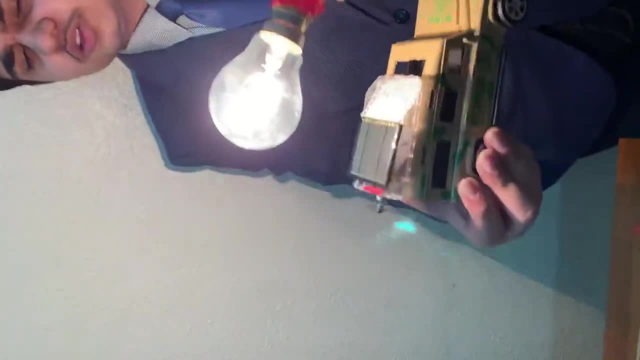 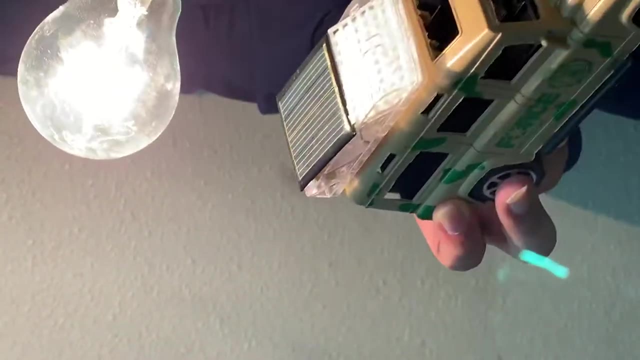 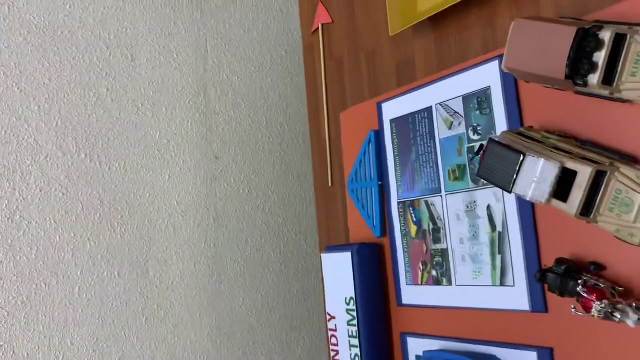 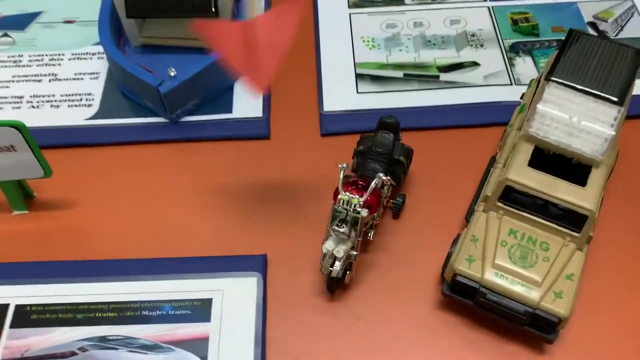 So you can see that As the light falls on the solar panel, The exhaust fan starts moving And sucks in the air, Thus purifying the air more and more efficiently. You can also appreciate the way These filters can be attached On the two wheelers. 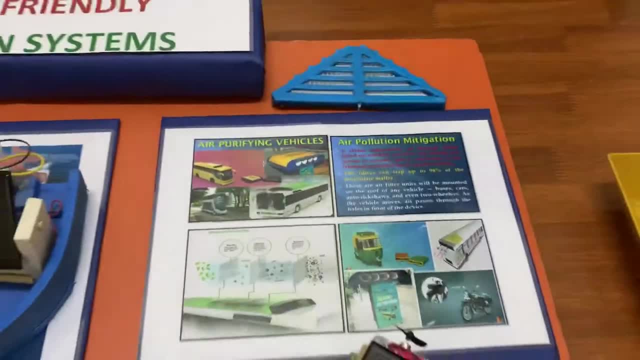 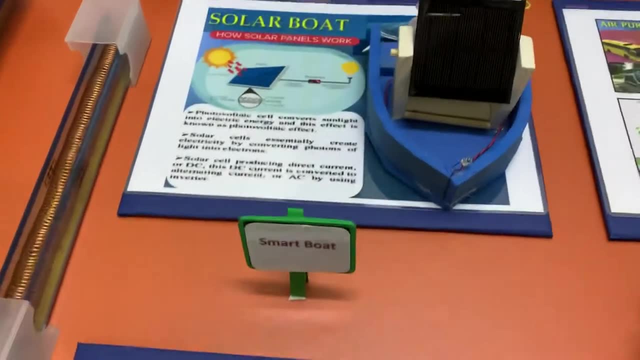 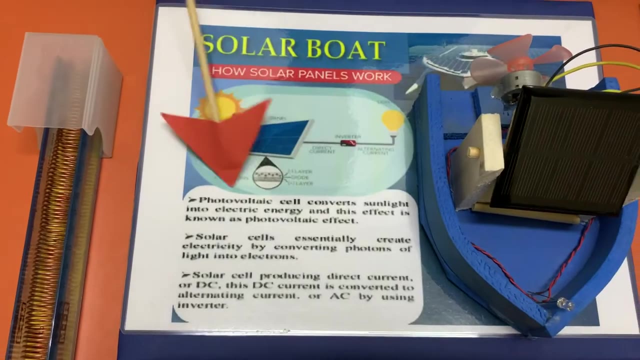 And the three wheelers Vehicles Now coming on to the solar board. This works. This board works on the principle of solar energy. Now, as the photons of the light fall on the solar panel, They knock down the electrons free from the shell. 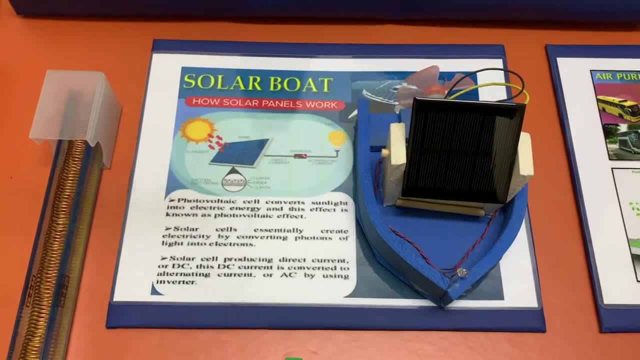 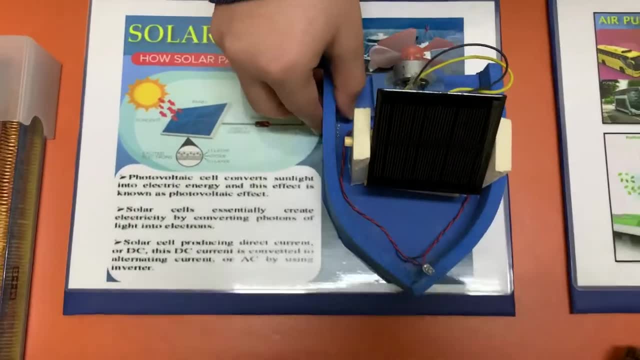 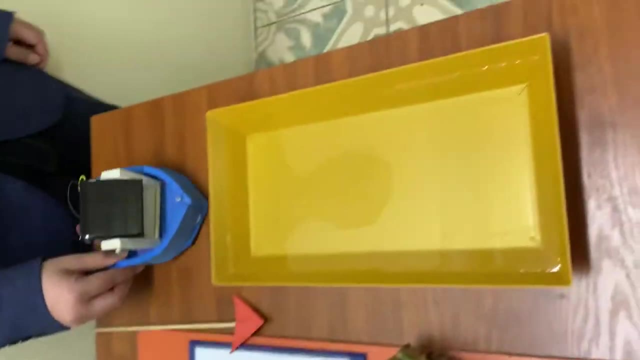 So these electrons starts moving rapidly And the flow of these electrons Produces electric current, Which powers our boat. Now you can see There are solar panels And DC motors attached to the boat. Now I'll demonstrate you the working of my boat.